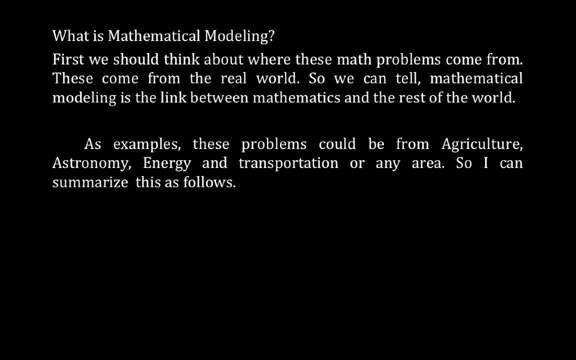 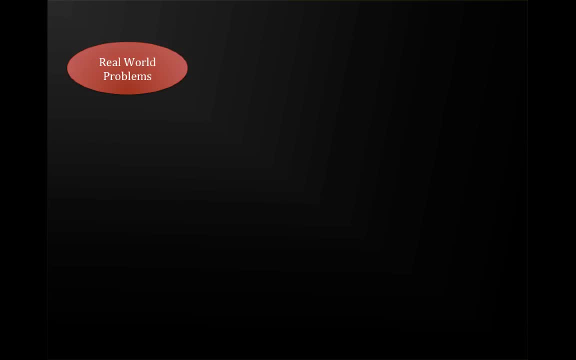 any area. So let me explain this mathematical modeling using some charts. So think about real world problems. Real world problems can be simplified to the real model, Then go to the mathematical model. Once we have a mathematical model, we can calculate and give a conclusions. 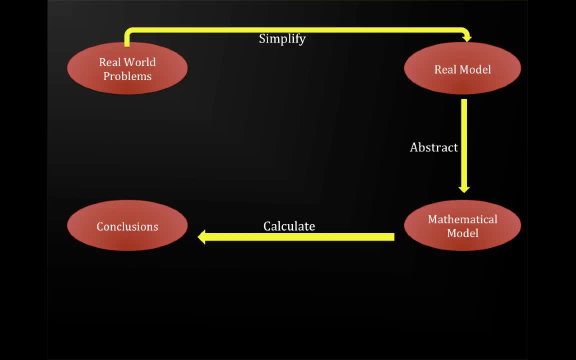 But most of mathematical models are complicated. How do we solve that type of models? Yes, we can use computer So we can write a program and make it a computer model. It means we gives our data into a computer, Then we can do the 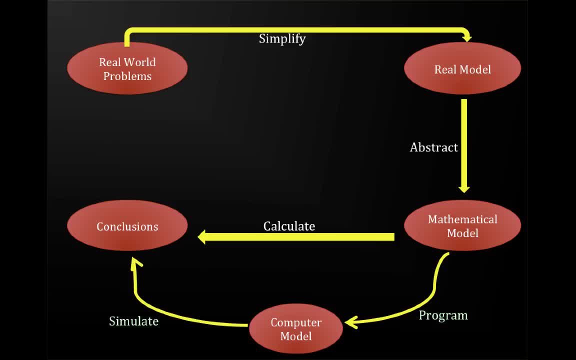 simulation and give a conclusion. So this is the easy path to solve the complicated problems, Then finally interpret. So in this course we are going to learn the techniques of these steps. steps Again: when you have a real work problems, you ask a question, You think a bit And then you refine the question. 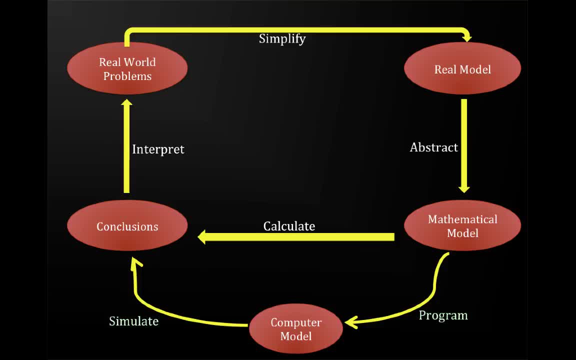 passing it in precise mathematical terms. Once the question is solved, its become a transcript. You continue to learn the process in talking about other functions. Somehow- this is not a typical- becomes a mathematics equation. you use mathematics to find an answer. Then, finally, you have to receive the process translating the mathematical solution. 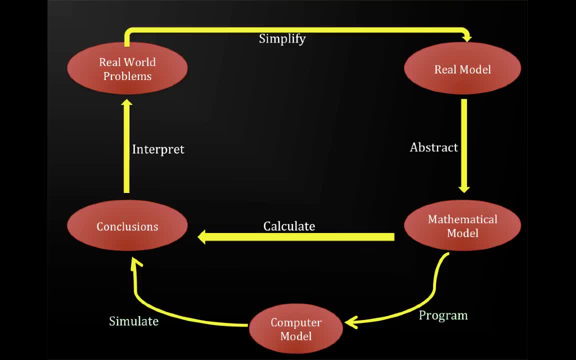 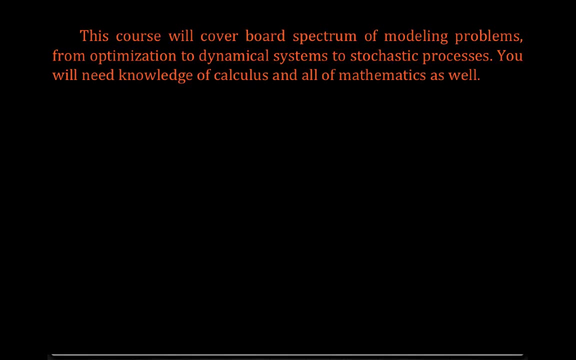 back into a comprehensible, no-nonsense answer to the original question. Now let me talk about the course. This course will cover both spectrum of modeling problems, from optimization to dynamical systems to stochastic process. You will need knowledge of calculus and all of mathematics as well. If you look at a few,